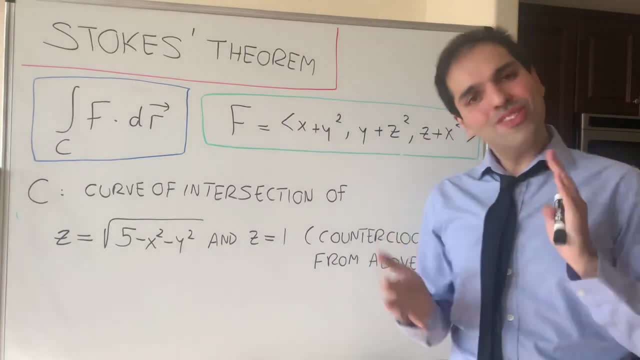 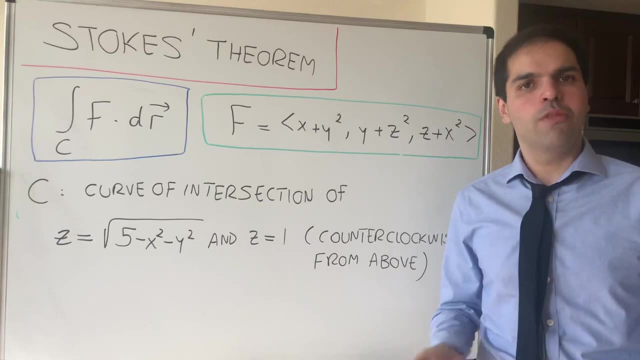 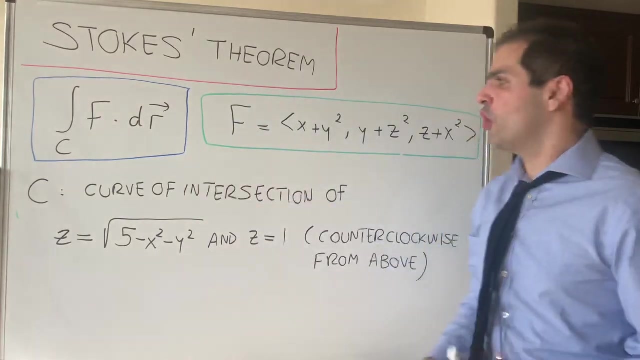 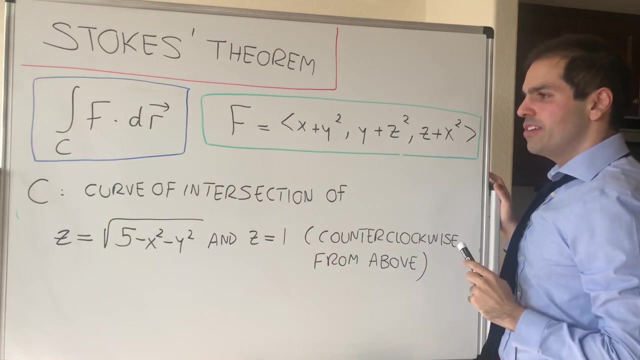 All right, let's get stoked with Stokes' theorem. So today I would like to present you the dark side of Stokes' theorem, where you use it to calculate a line integral instead of a surface integral. And in fact, today we'll calculate the line integral of f- dr, where f is this adorable vector field x plus y squared, y plus z squared, z plus x squared, and where c is the curve of intersection of two surfaces. 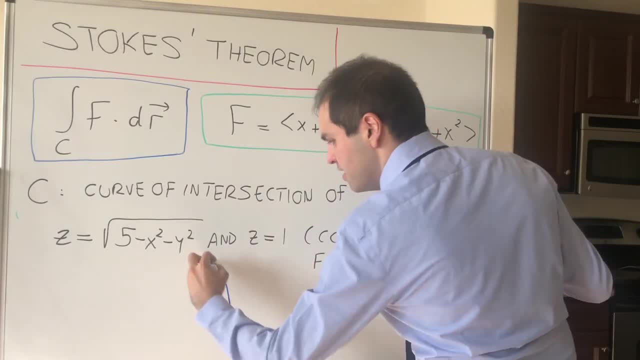 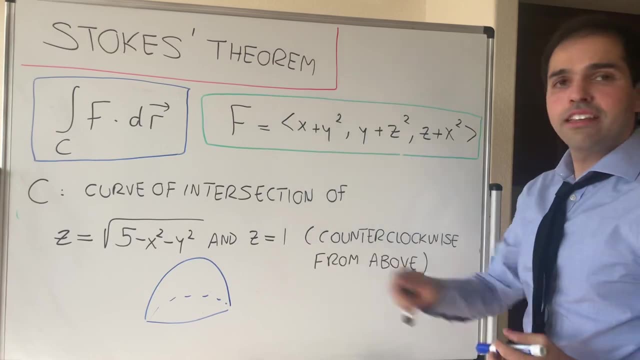 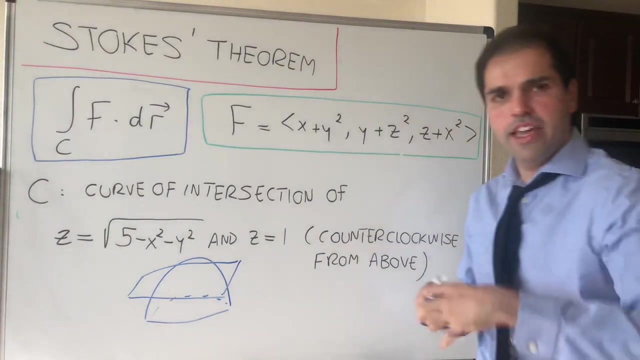 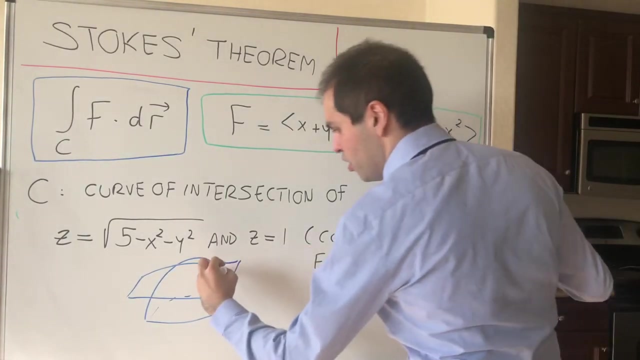 On the one hand, the hemisphere z equals square root of 5 minus x squared, minus y squared, and the plane z equals 1.. So what this surface is? you simply take a hemisphere and you cut it off by a plane and we'll show later that in fact this is a circle, and this circle we'll call it c. 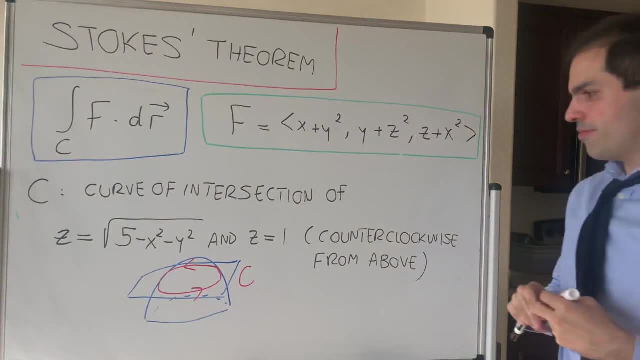 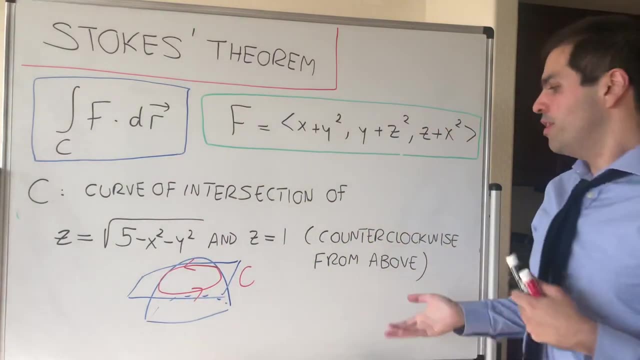 Again, claro que c. And what we would like to do? we would like to calculate the line integral of f over this circle, and orientation matters here. So we orient it. We orient it counterclockwise if you look at it from a bird's eye view. 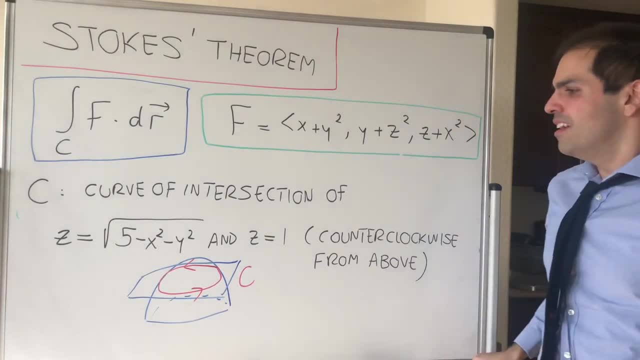 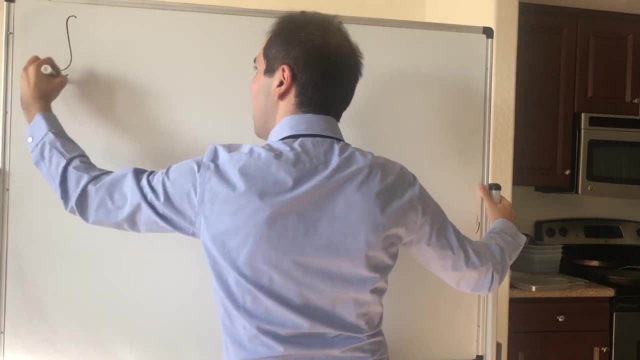 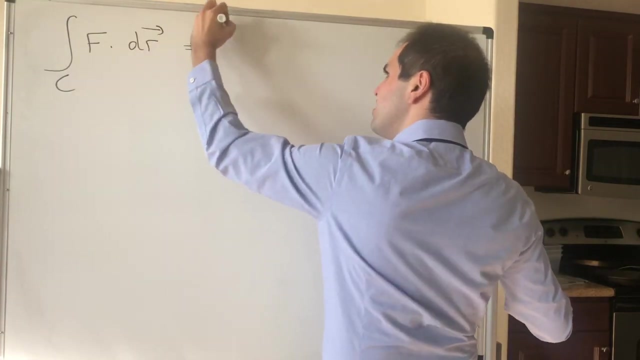 So if you look at it from above, it is counterclockwise. All right, and so what does Stokes' theorem say? It simply says the following: It says that the line integral of f- so the stuff we want to calculate- is just the same thing as the surface integral of the curl of f. 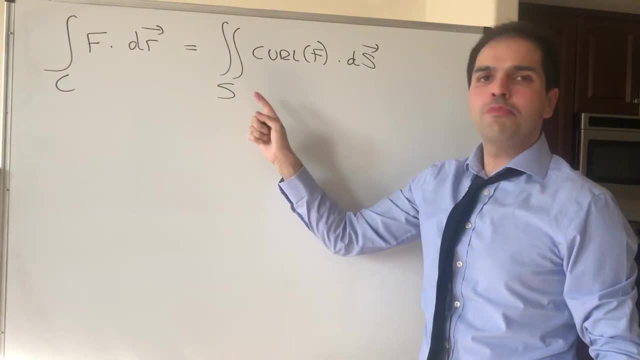 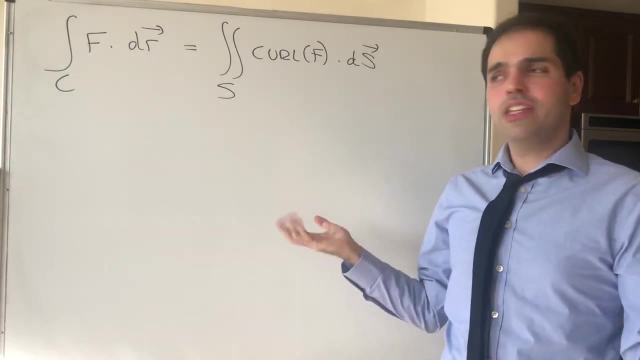 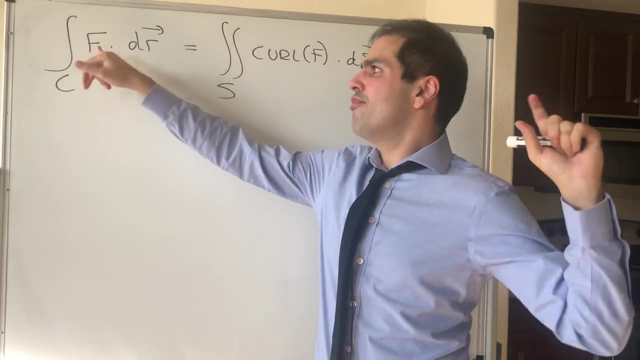 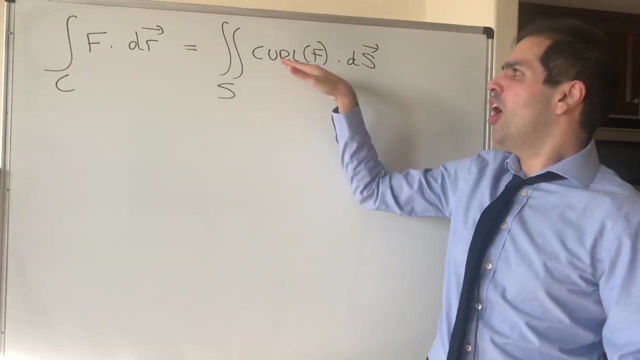 In other words the integral. The integral of a function is the same as the double integral of a derivative. So it is like the fundamental theorem of calculus, but here what it says is simply the following: The line integral, so an easy integral of a complicated function, becomes a surface integral, so a complicated integral of an easy function. 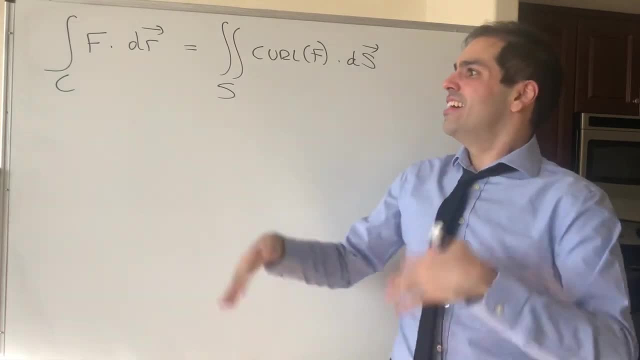 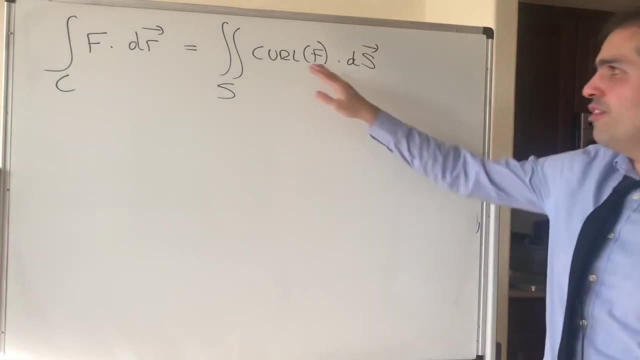 So in some sense this is the yin-yang of math: Easy of heart, It becomes hard of easy. so it can't balance this out. And for this now, the first step is of course to calculate the curl of f. 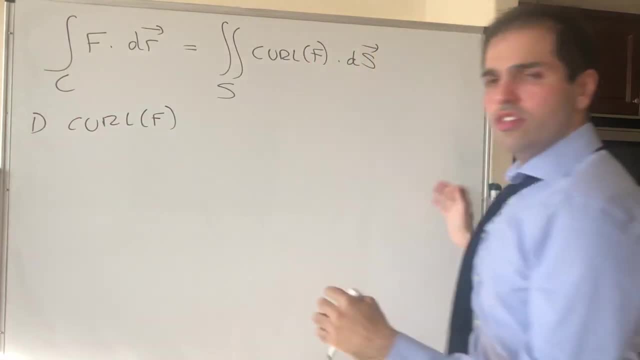 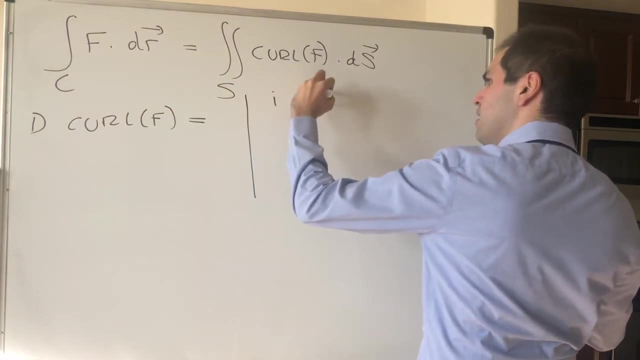 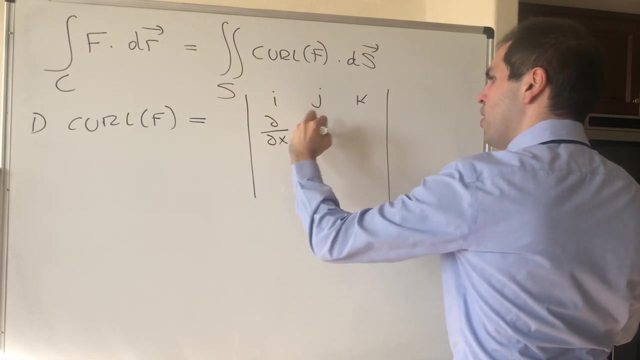 So the curl of f, I'd like to remind you, is just a gradient crossed with your vector field and what it becomes is just a big determinant ijk of, again, partial over partial x, partial over partial y, partial over partial z. 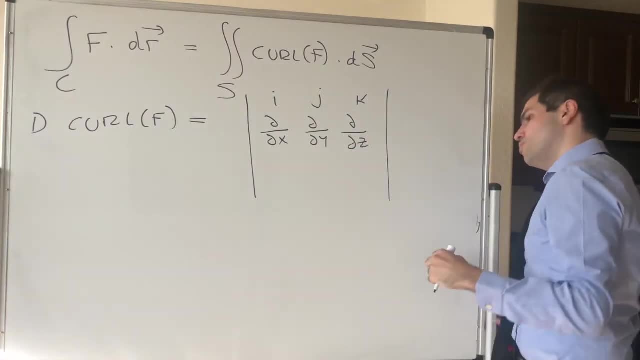 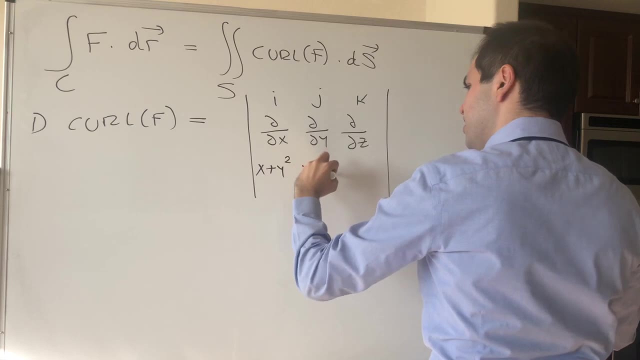 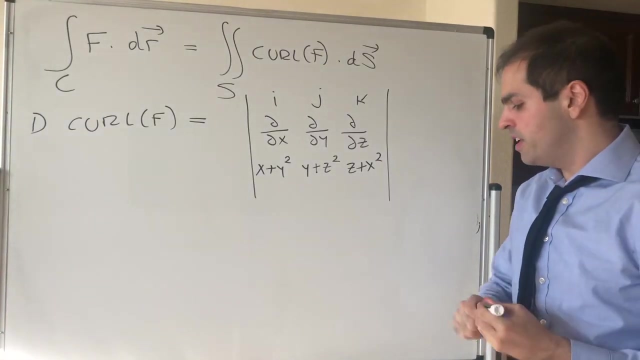 and you put your vector field, so which, I'd like to remind you, is just x plus y squared, y plus z squared, and then z plus x squared. So all we need to do is to calculate this determinant. So let me remind you how to do this. 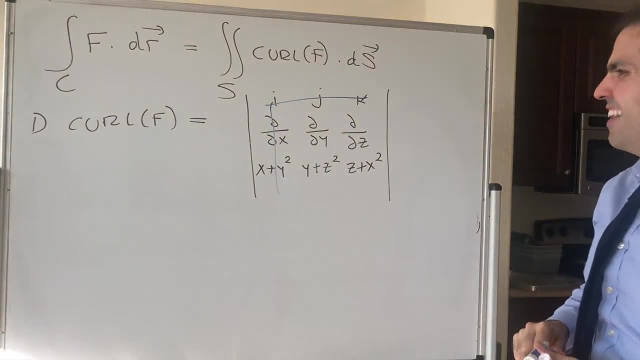 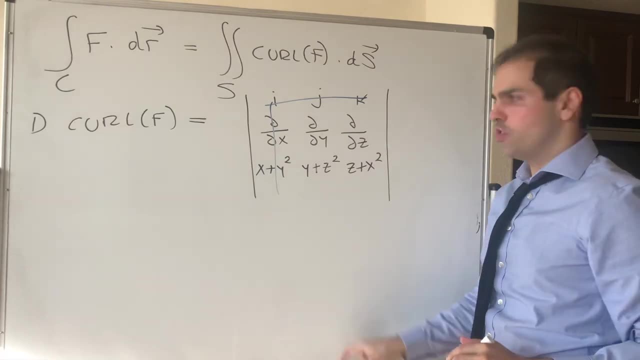 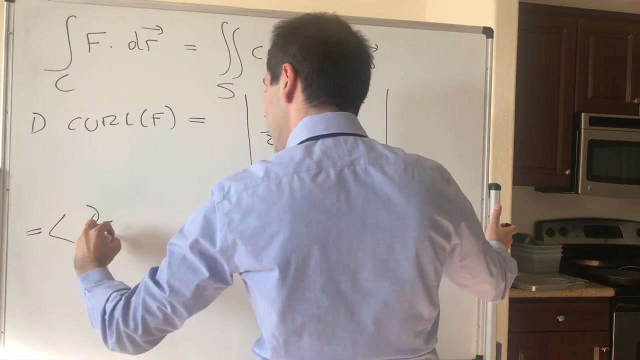 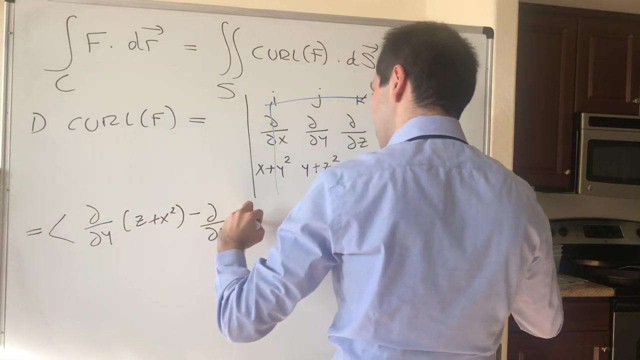 So you start with the first component And bomberman this. what you get is simply partial over partial y of that, minus partial over partial z of this component. Let me write that down. So partial over partial y of z plus x squared, minus partial over partial z y plus z squared. And then the 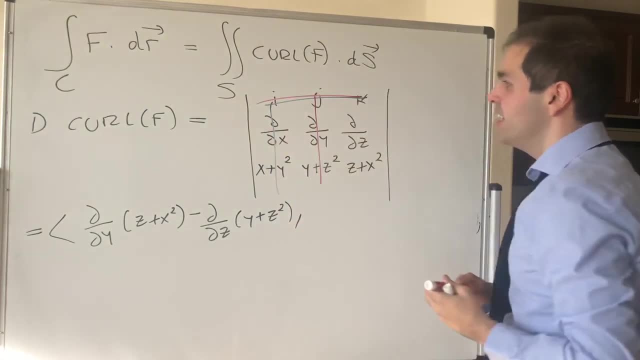 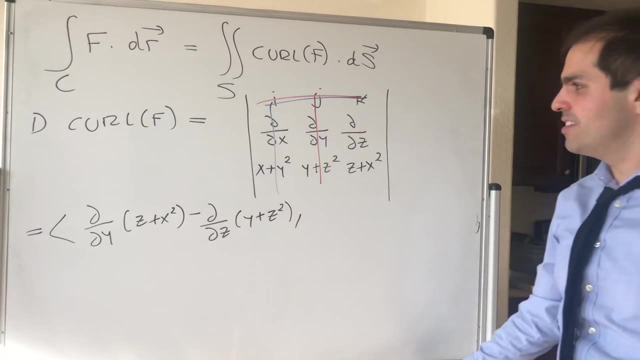 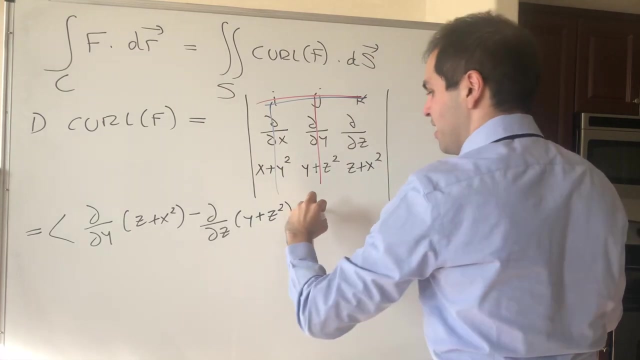 second one, this one in red, remember because you're doing the terminance. it becomes plus minus. so there's this minus thing here, and what this becomes is not this times this, but minus this times this. so minus, partial over partial, x z. 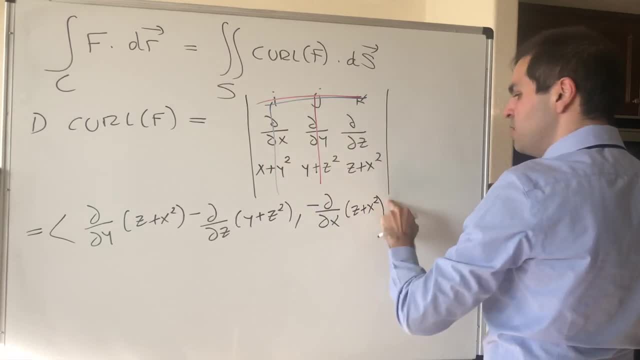 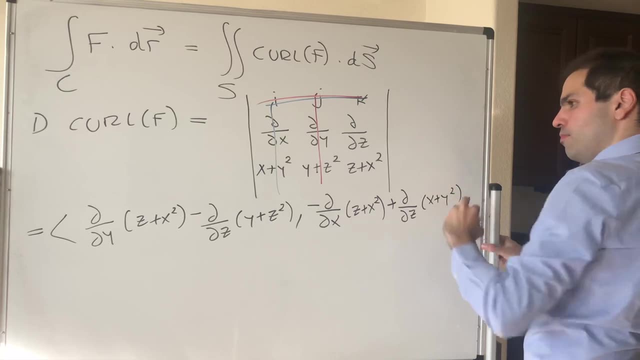 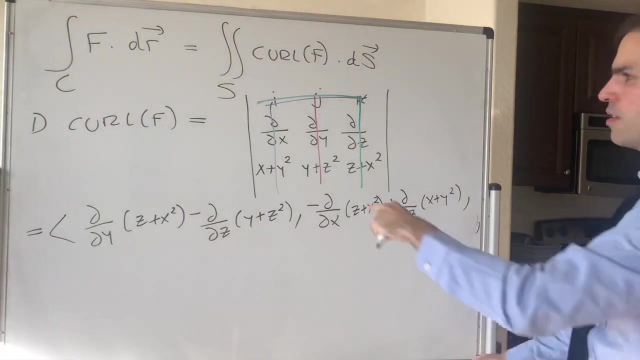 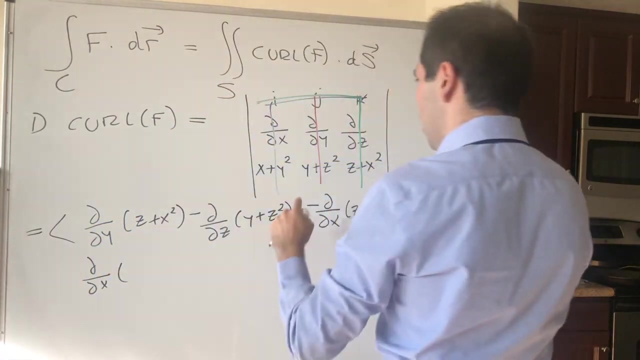 plus x squared, and then minus minus becomes plus, so plus partial over partial z, x plus y squared. And last but not least, we have the very last component, this one here which becomes partial over partial x of this, so partial over partial x of sorry of this, sorry. 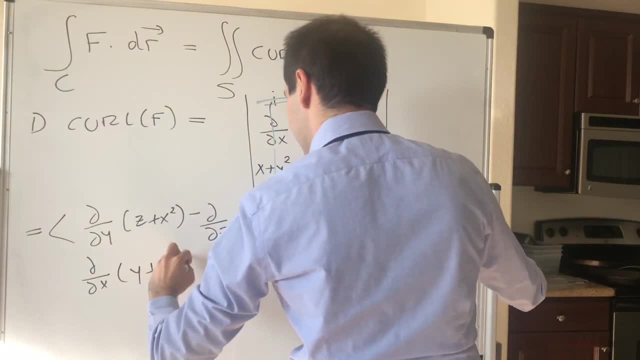 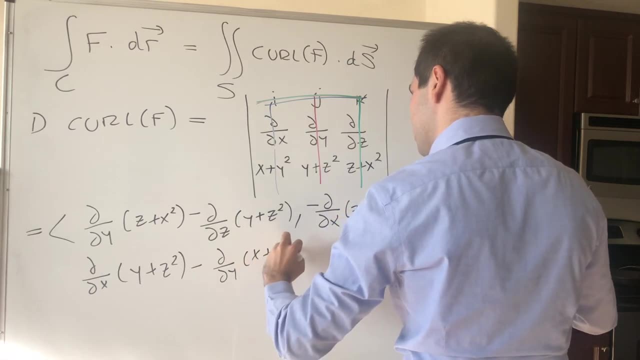 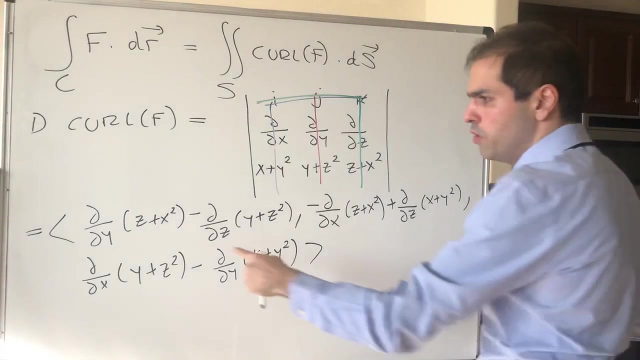 of y plus z squared, minus partial over partial y of x plus y squared. Now I know this looks complicated, but look it simplifies so beautifully. This thing disappears because there is no y. This thing just becomes minus 2z. 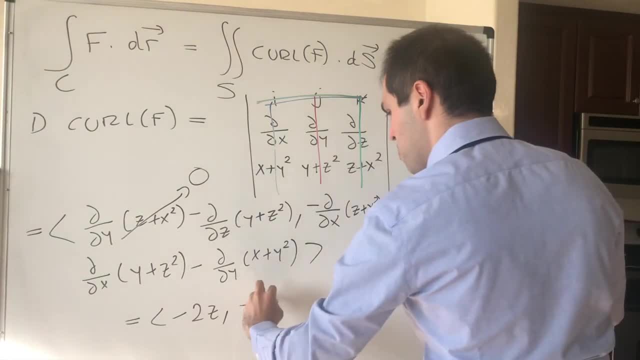 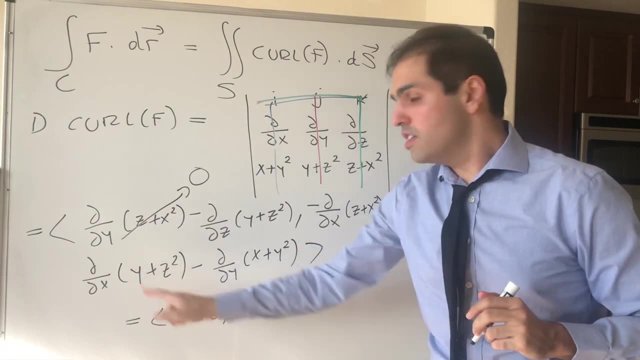 Now this thing becomes minus 2x and this disappears Again. you're the weakest link, goodbye. And then this disappears because there is no x. And last but not least, we have the partial over partial y of x squared. 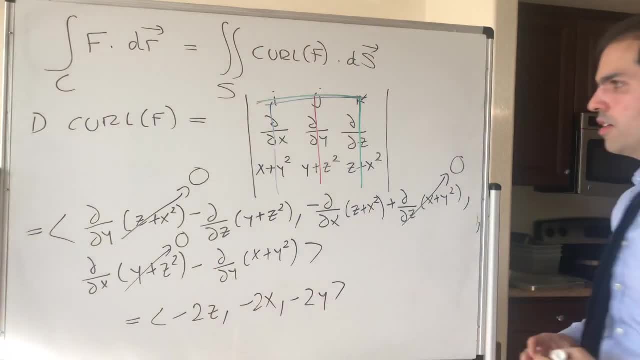 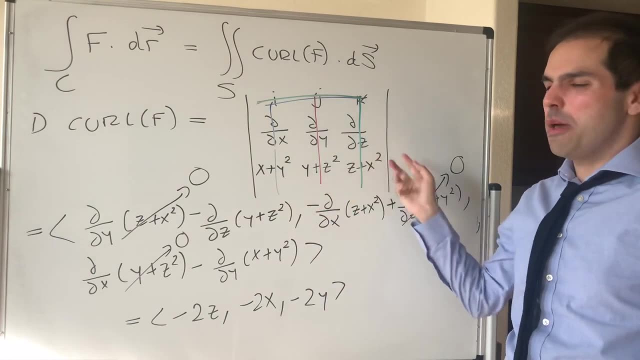 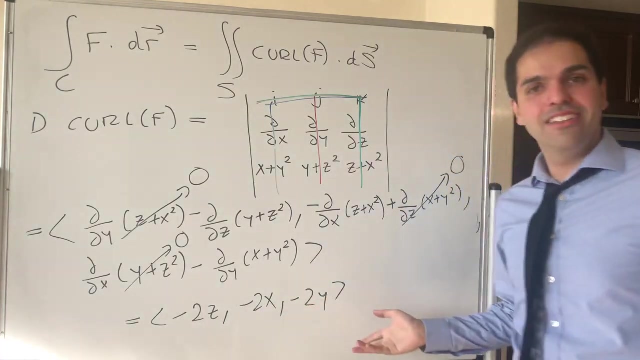 And last but not least, we have the partial over partial y of x squared And after you get minus 2y. So let me ask you this: which is easier to integrate: x plus y squared, y plus z squared, z plus x squared, or, hmm, minus 2z, minus 2x, minus 2y? 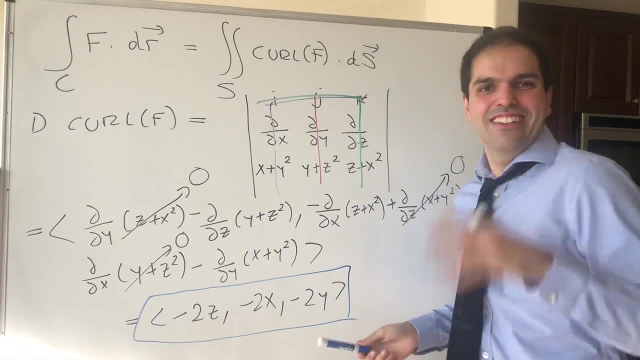 It's like this meme of this person that's like ugh, you know, sounds disgusting, but now this is more and more. It's like this meme of this person that's like: ugh, you know, sounds disgusting, but now this is more and more. 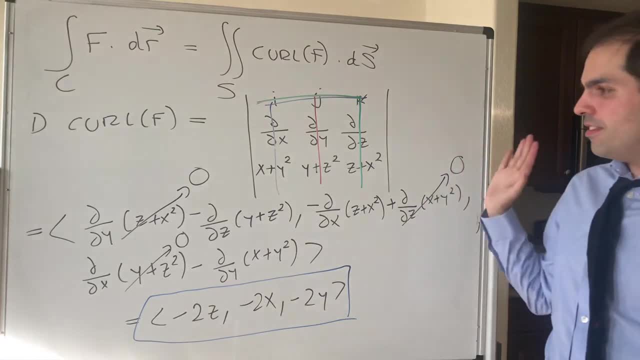 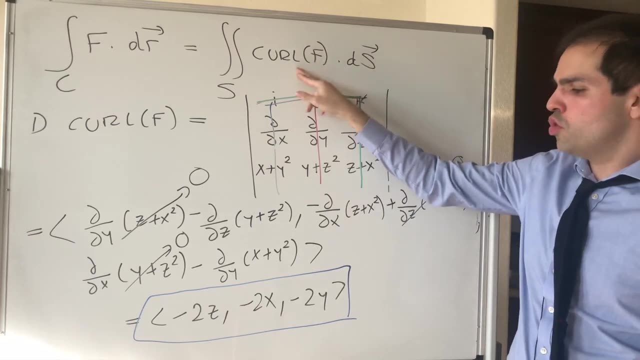 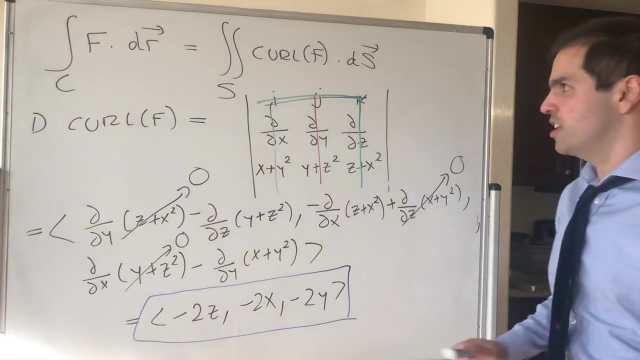 delicious, yeah, All right. So all we need to do again, instead of doing a line integral of this hard thing, you just need to do the surface integral of this easier thing. So win-lose situation. but now the next question is: what is the surface? 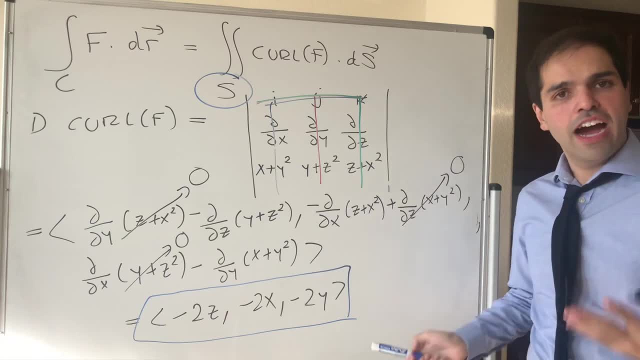 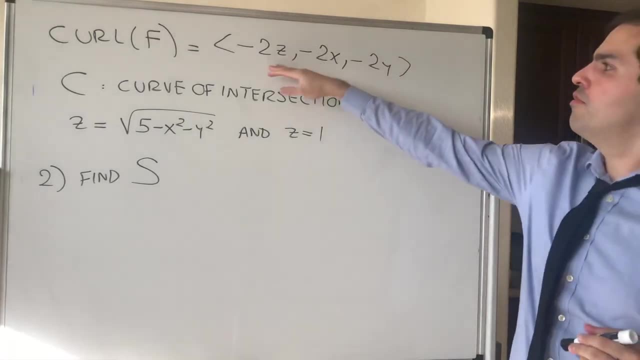 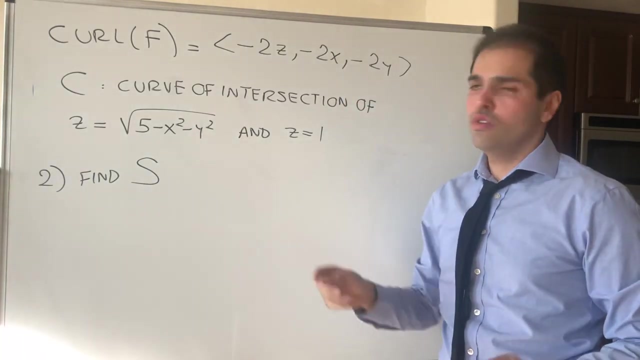 What is this? And for this, let's figure out first of all what the curve is. All right, so again, let me remind you. All right. so again let me remind you, the curl of f was this easy vector field and c, from the very beginning, was just a curve of intersection of those two surfaces. 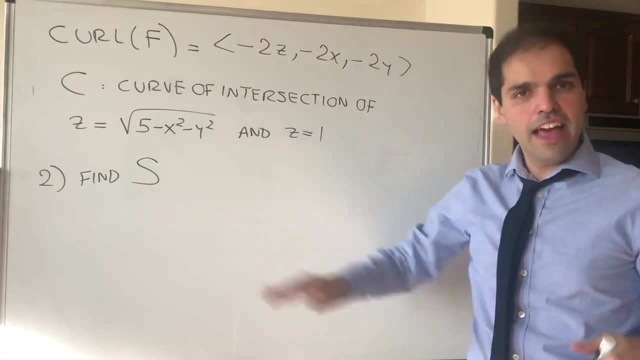 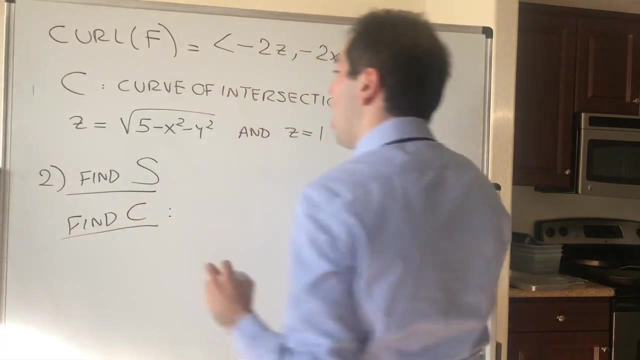 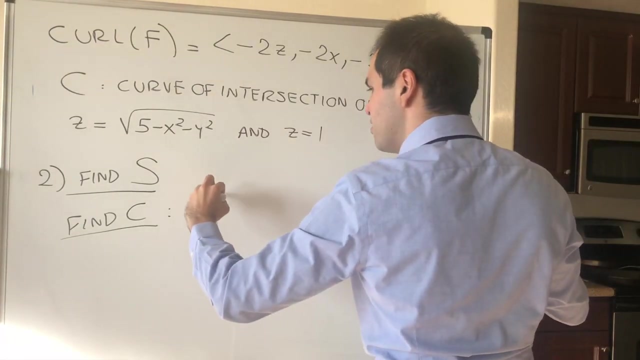 So, as I said, our goal is ultimately to find s, but before we do that, let's first of all find a curve, Find c, but that's not very hard, because all you need to do is intersect those two things. so that set this equal to this. so square root of 5 minus x. 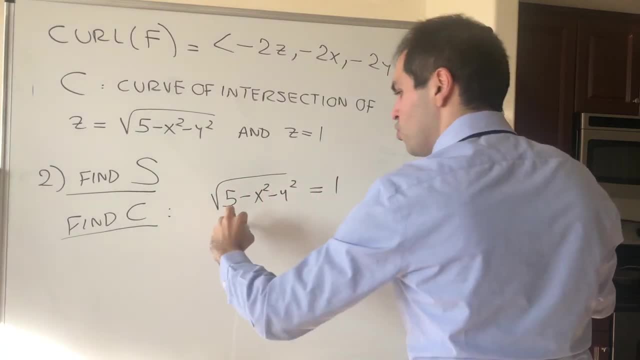 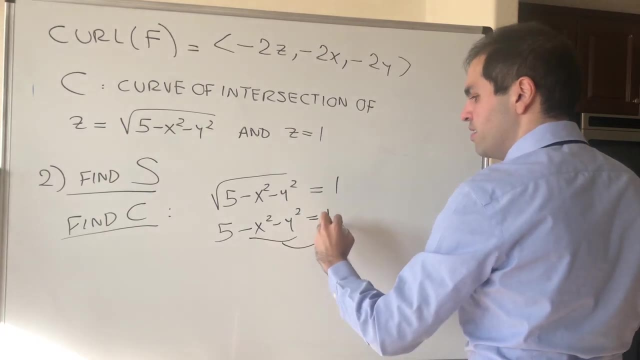 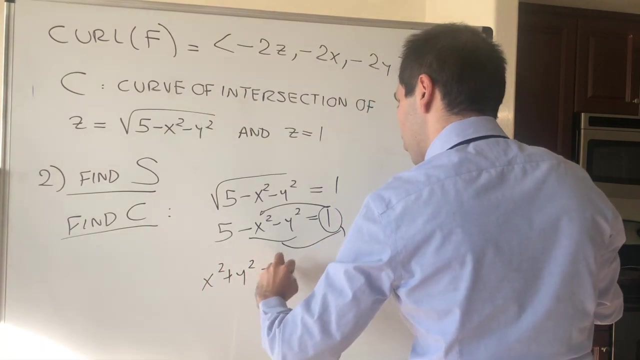 square root minus y squared equals 1, and then we get 5 minus x squared minus y squared equals 1, and if you put this on the right-hand side and this on the left, you ultimately get x squared plus y squared equals 4.. 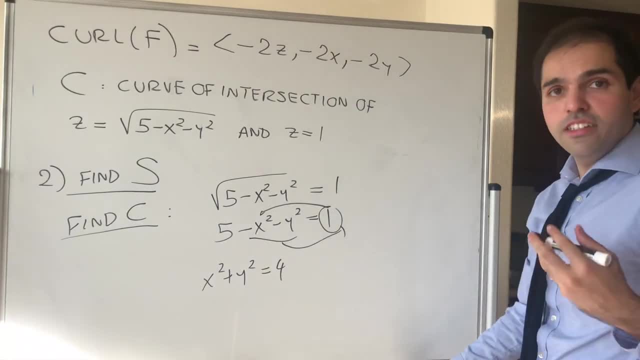 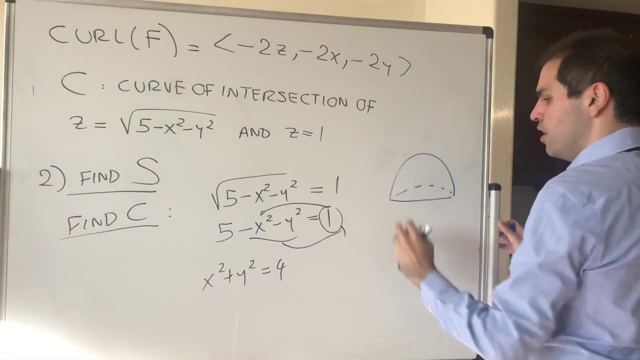 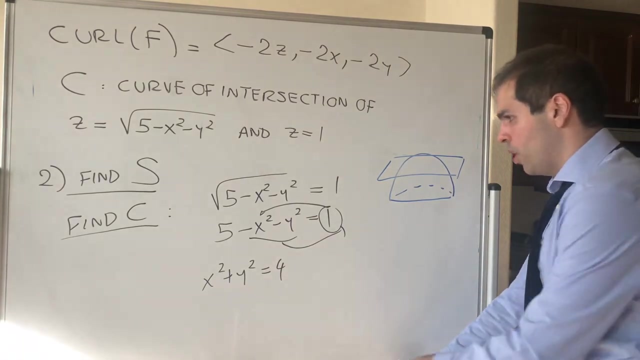 So what this is is that c is a circle. okay, it's a circle of radius 2, but just be a little bit careful: it's not the, It's not the one in the x-y plane, it's the circle in the plane. z equals 1.. 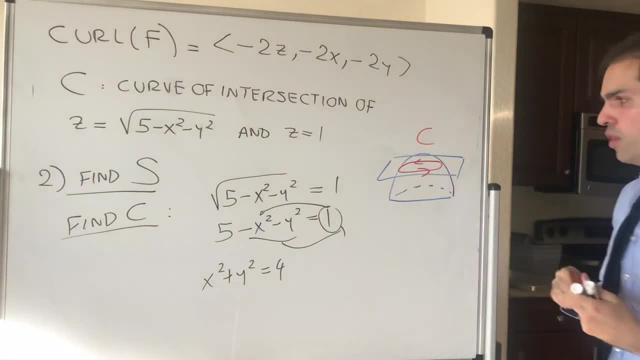 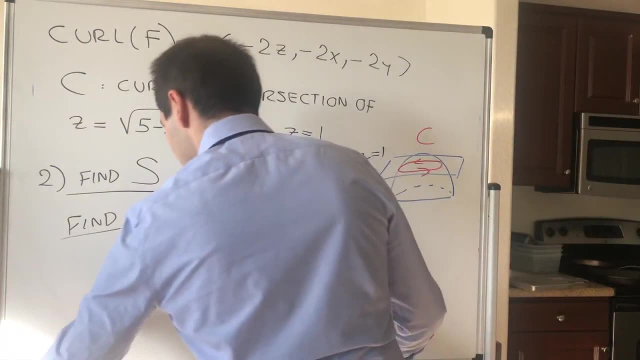 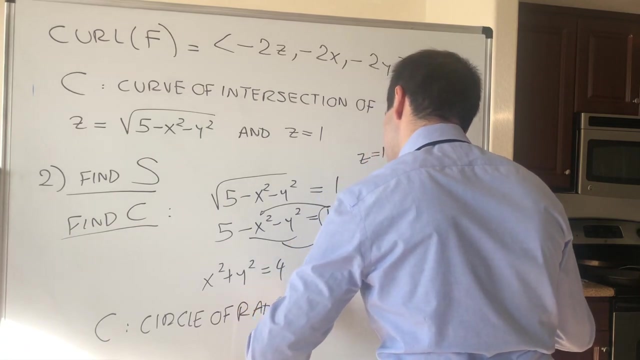 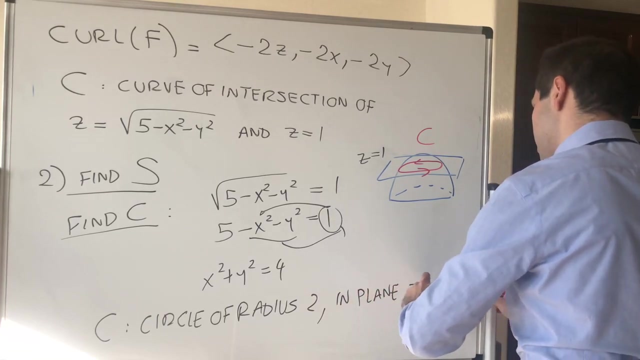 So again, just like our picture showed, c is a circle, but in the plane z equals 1.. So c is again just a circle of radius 2 in the plane z equals 1.. Now here's the thing. the question is, what is the surface? 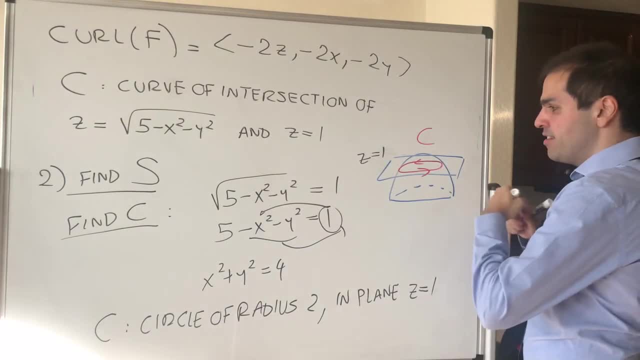 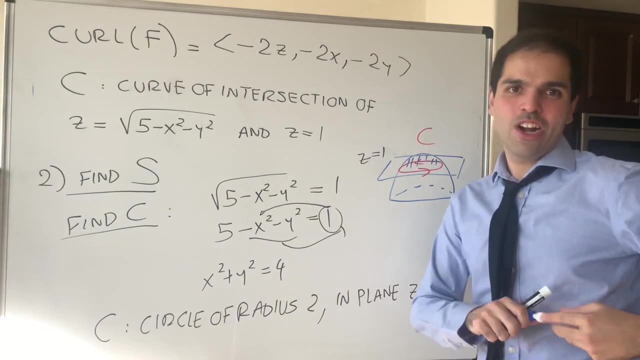 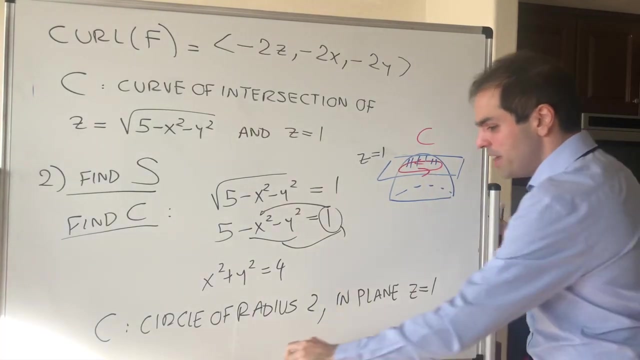 You might be tempted to just say s is just the upper hemisphere, and then parametrize the upper hemisphere and then cry because you would have to do, you know, cross products, etc. etc. but actually none of that thing, because 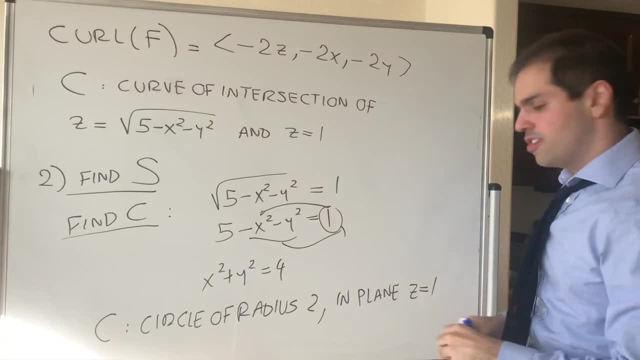 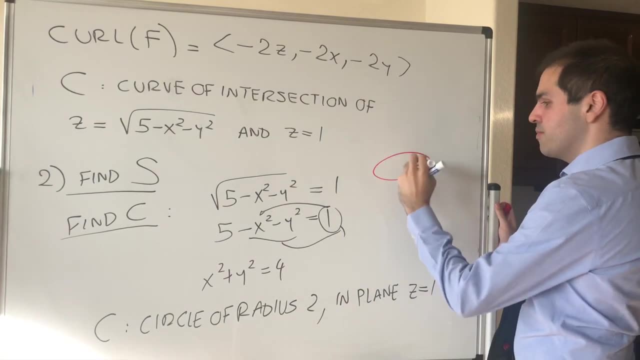 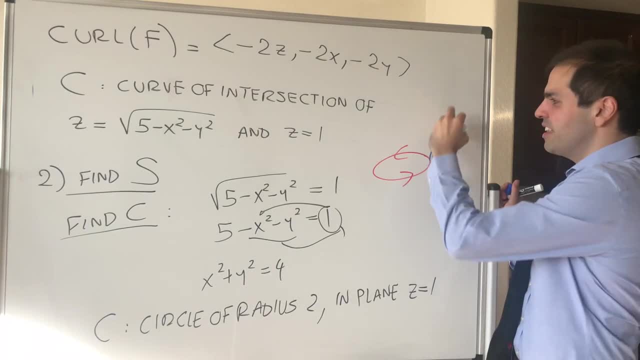 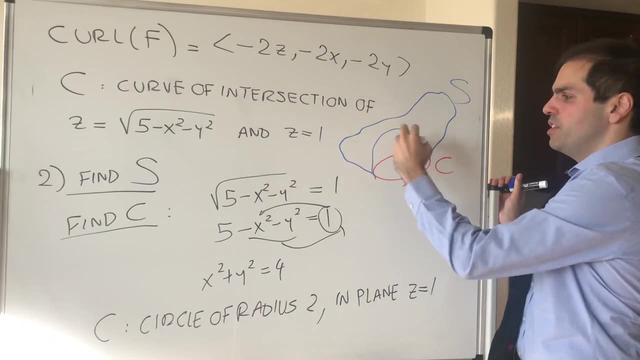 if you want to orient it upward or something, you still get the same result. So you could pick s to be this weird surface, You could pick s to be the hemisphere, or you could even pick s, or you could even pick s. 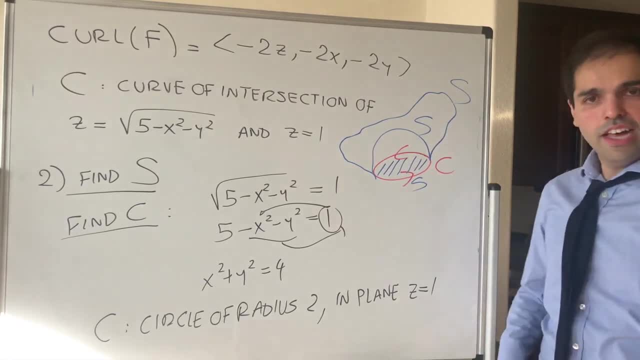 or you could even pick s to just be the inside of that circle, or you could even pick s to just be the inside of that circle, or you could even pick s to just be the inside of that circle. It would all give you the same result. 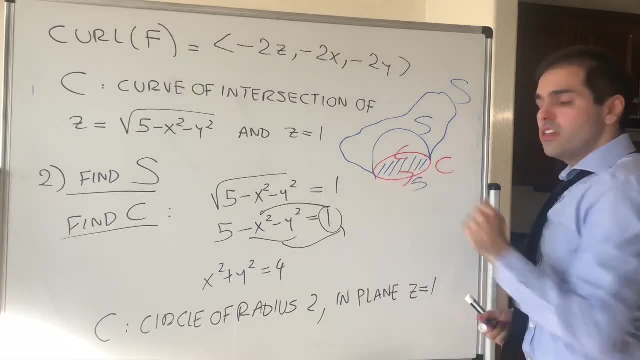 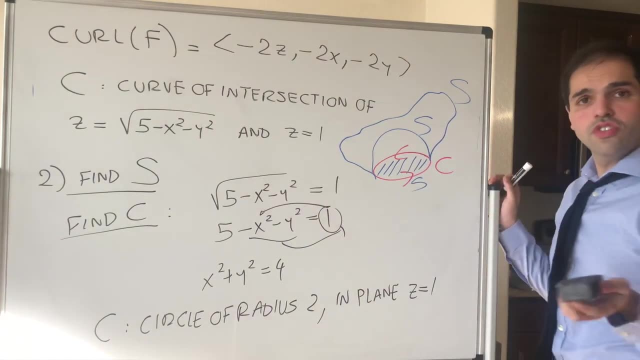 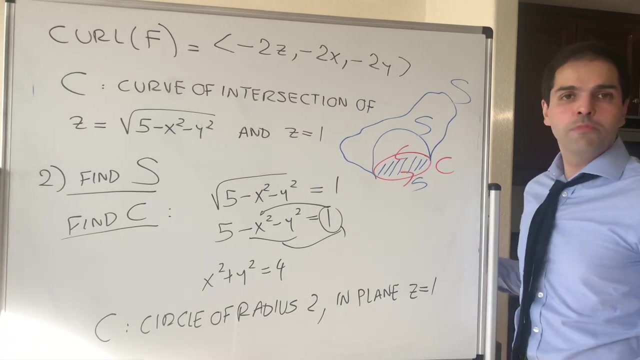 So why not just be lazy and pick the easiest version, which here is? just this flat surface. So again, just to re-iterate what is s Well, because the result doesn't depend on which surface we have, let's just pick the easiest one. 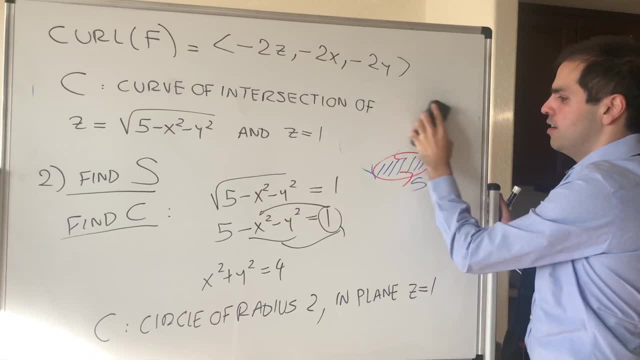 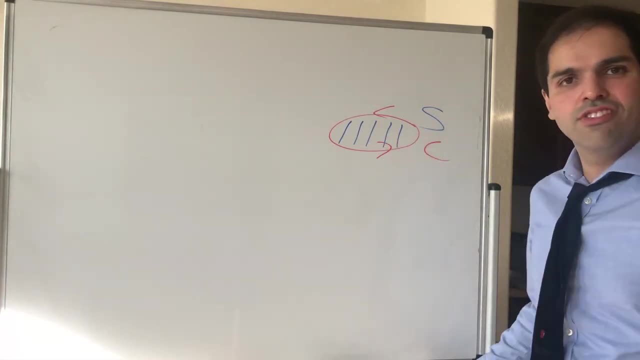 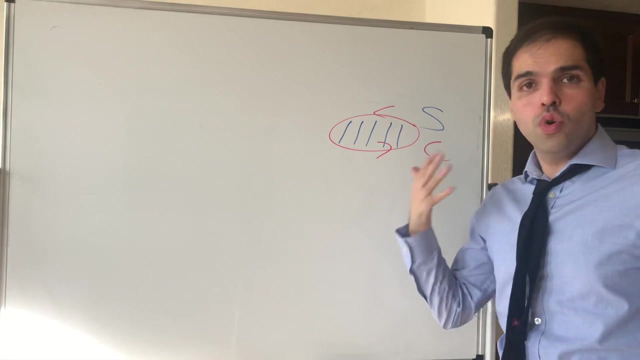 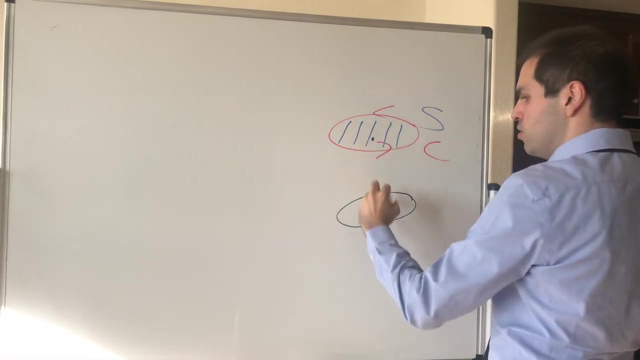 which is just the inside of this circle. alright, so now that we figured out that it's the inside of the circle, the question is: how do you parametrize it? well, here you have many different choices. you could use polar coordinates, or even lazier, just pick xy. so if this is xy, this surface is just. 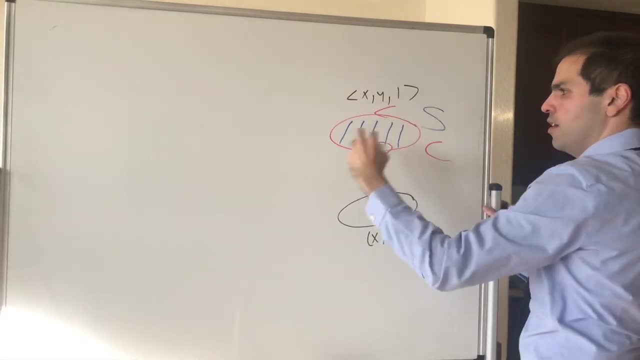 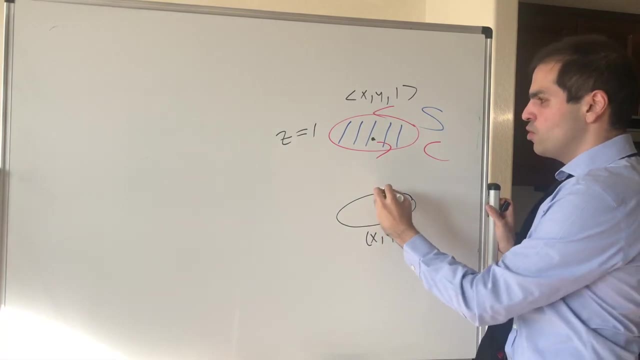 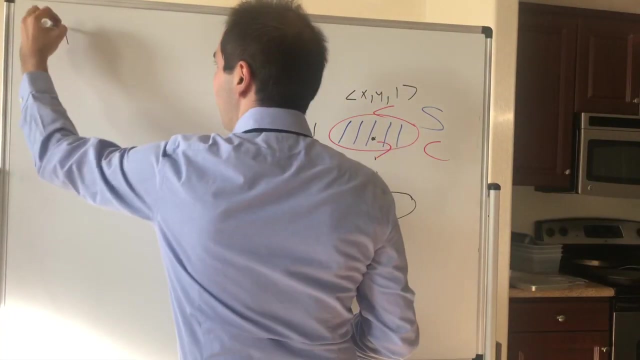 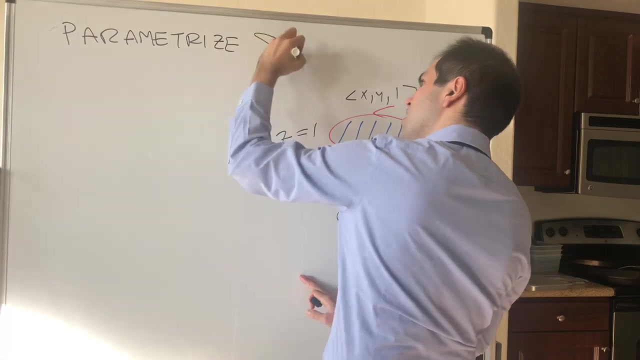 parametrized by xy and 1 because remember, this is in everything is in the plane. z equals 1, so kind of the shadow is xy. but if you go up you can just parametrize this with xy comma 1. so parametrize s, and so simply we just choose r of xy to be xy comma 1. 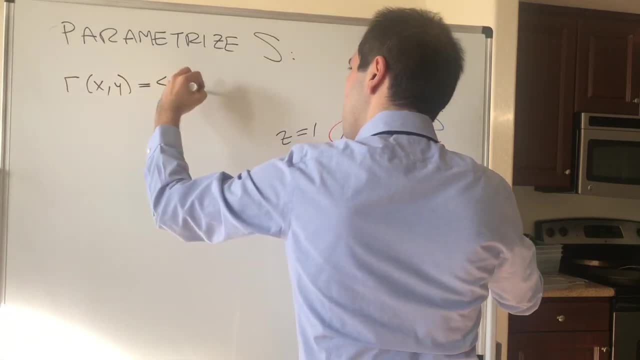 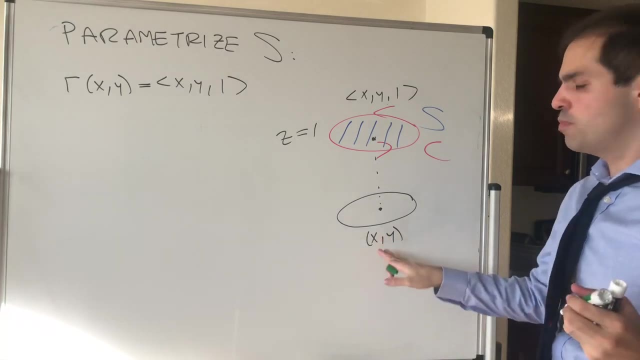 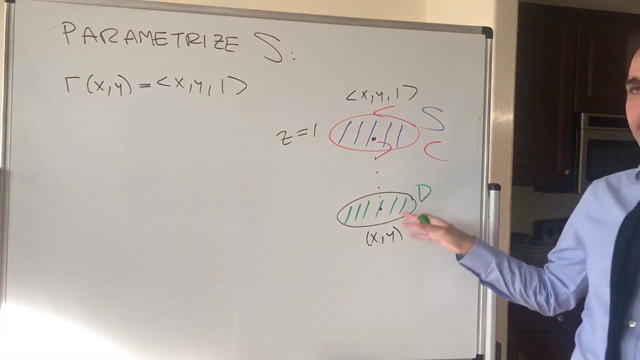 and, by the way, very soon I will write d. well, d what it is. it's just a space where x and y lies in, and in this case, what it is, as we found, it's just a disk of radius 2, in other words the shadow under s, and so the question is then: well, 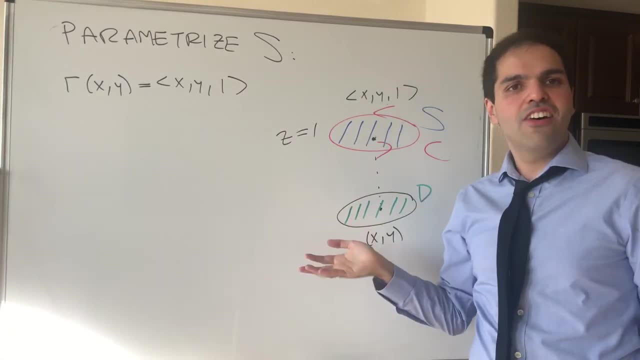 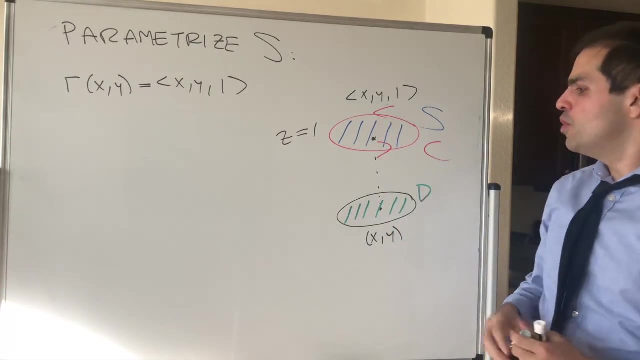 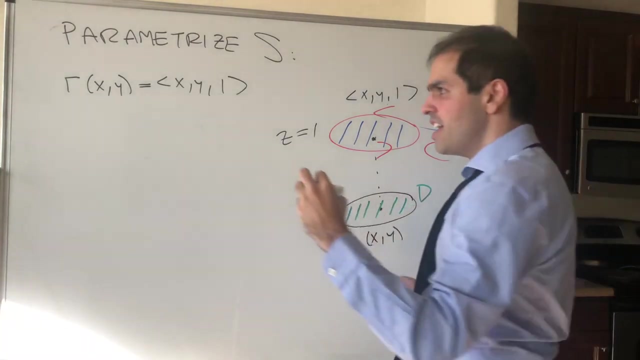 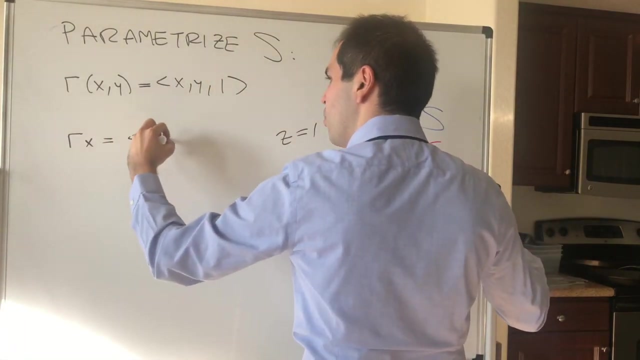 now that we found a parametric parametrization, how can we calculate the surface integral? remember, it's just finding the outward pointing normal vector, which you can just get by calculating the derivatives of r and crossing them. so let's calculate rx, so you just take the x derivative of each component. so 1 0, 0, you calculate ry. 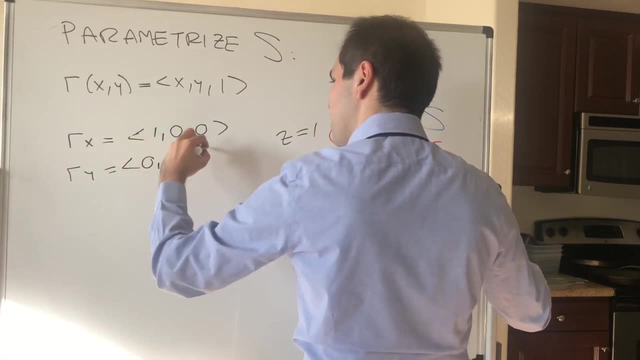 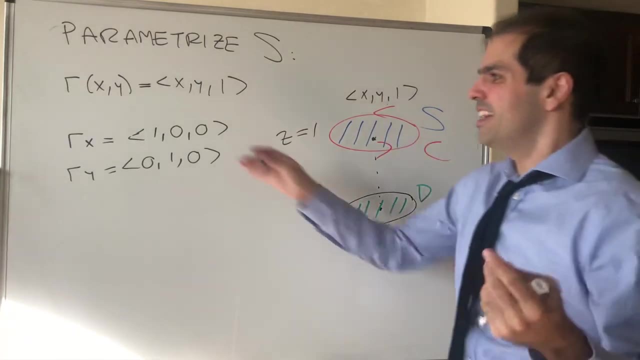 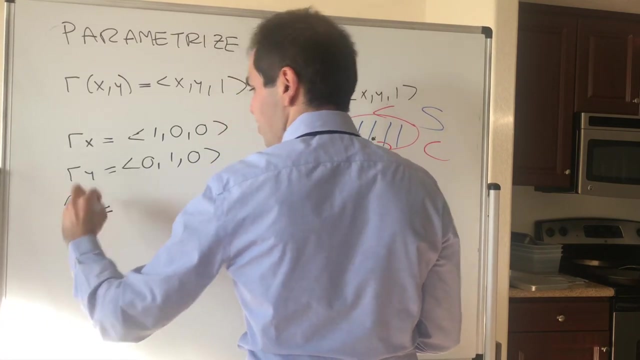 which is 0, 1, 0, and then you cross them. I know physicists are like: obviously it's k, but just in case you have a harder problem, at some point you calculate the normal vector. so let's, I called it n hat, which is rx cross ry, and that becomes again. 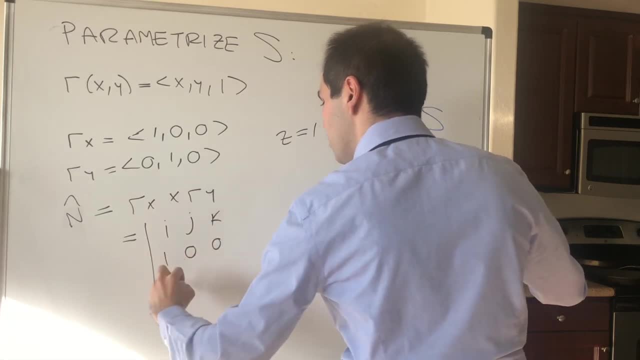 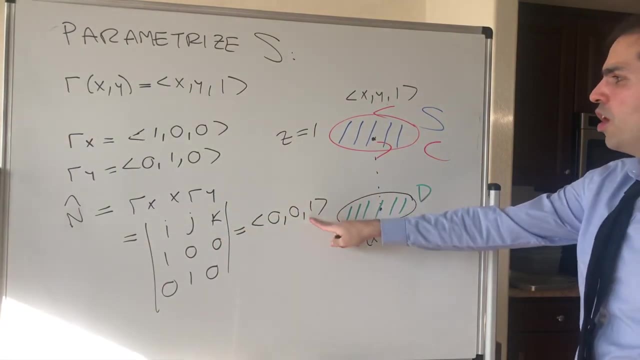 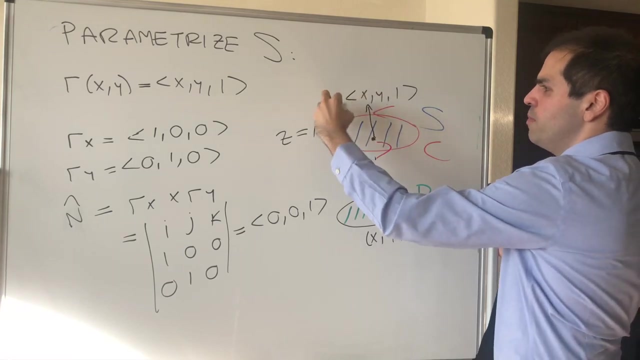 ijk 1 0, 0, 0, 1, 0 and we get in the end 0 0, 1. but remember you always need to check if the orientation makes sense. so here, if the curve is counterclockwise, you need to make sure that the normal vector faces up and 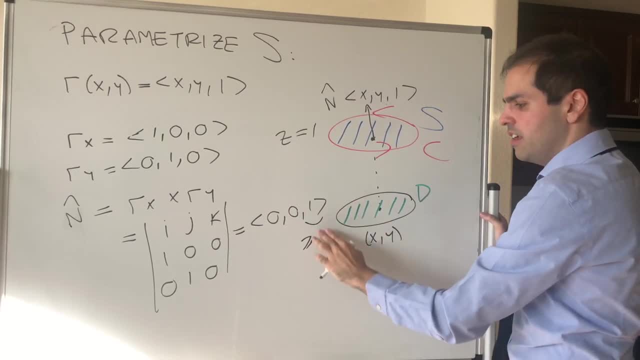 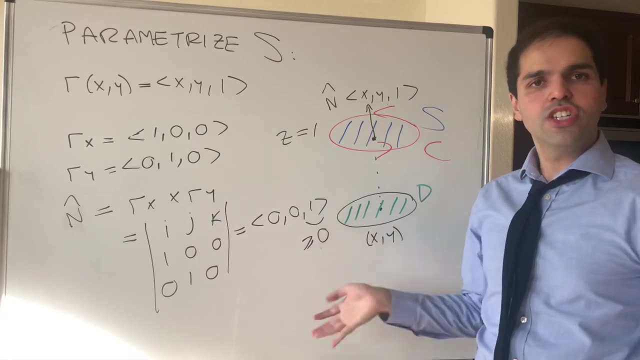 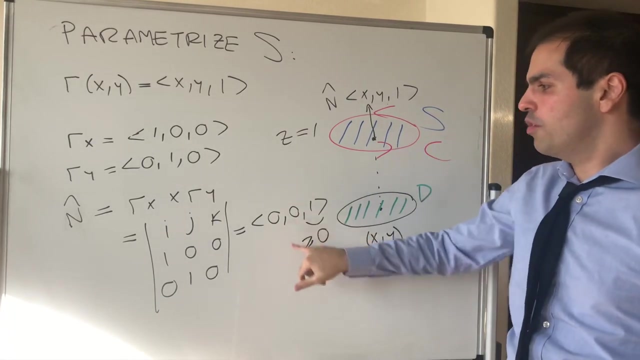 indeed it faces up because the last component is non-negative. I guess it's positive in this case. so this is the correct normal vector. and then the question is: how do you evaluate the surface integral? well, you just take your curl and you dot it with this normal vector. 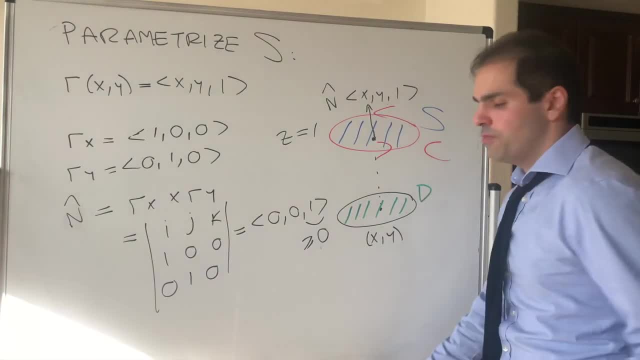 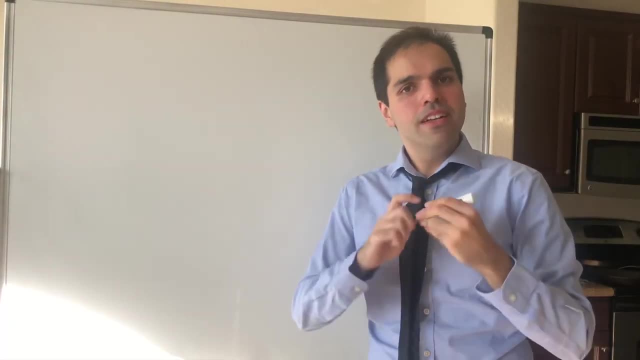 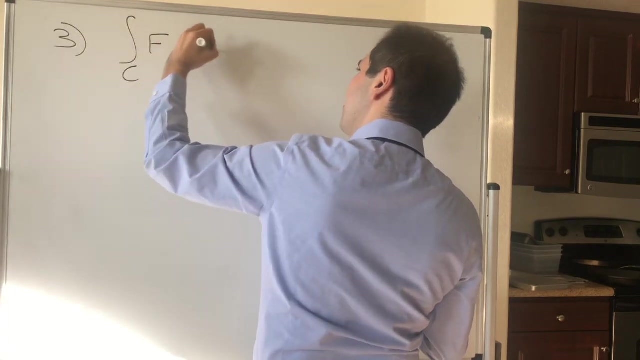 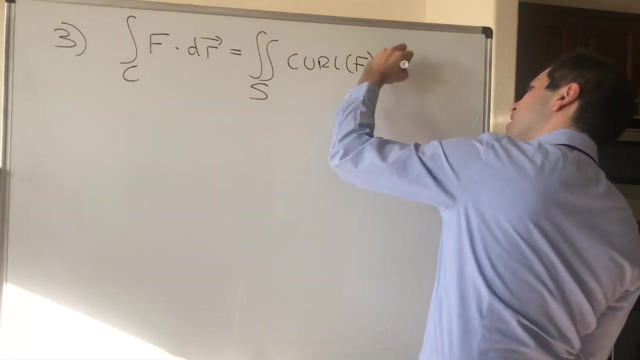 and you integrate the resulting thing. so, last but not least, we arrived at our final step. all right, and now we've just arrived at our final step. so let's actually calculate the line integral. so remember, by Stokes theorem, the line integral of f is the same thing as the surface integral of the curl of f dotted with ds. 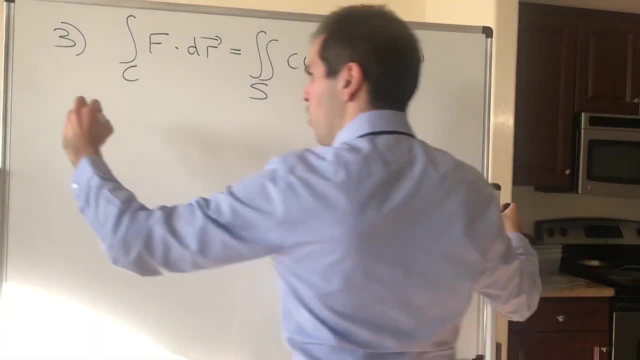 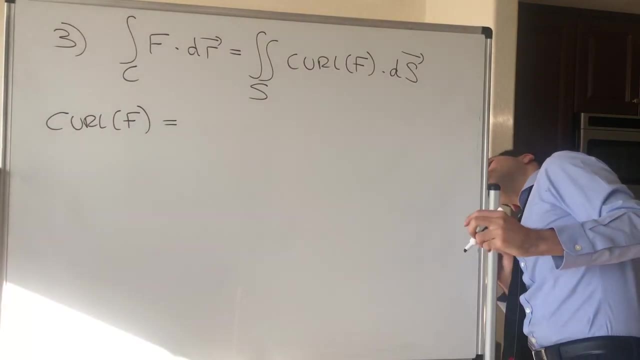 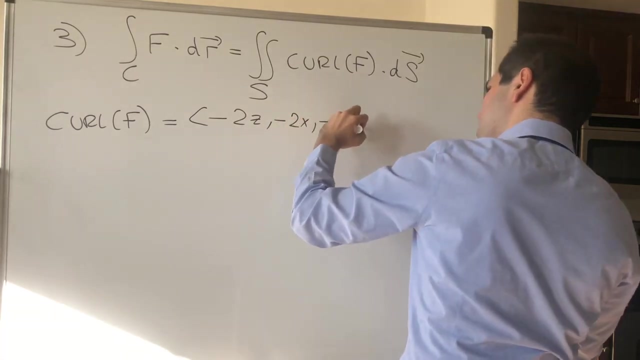 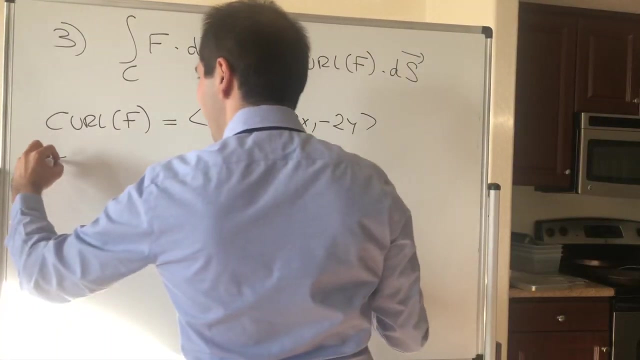 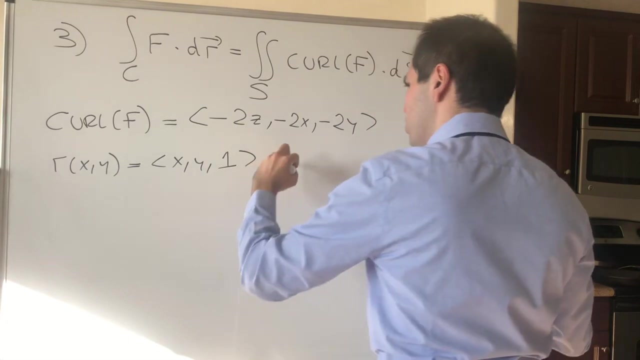 now I would like to remind you the curl was this easy vector fill. that was just- I keep forgetting- minus 2z, minus 2x, minus 2y and we had this parametrization. so rxy equals xy1 and the normal vector was just. 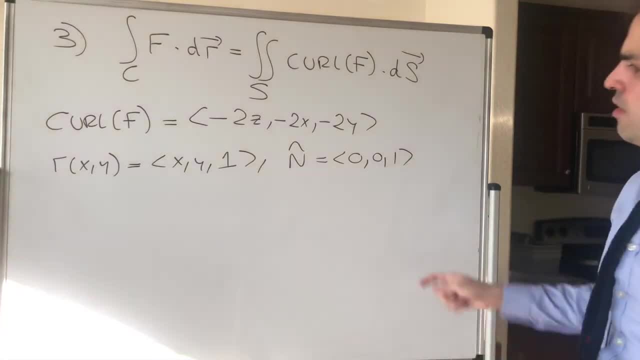 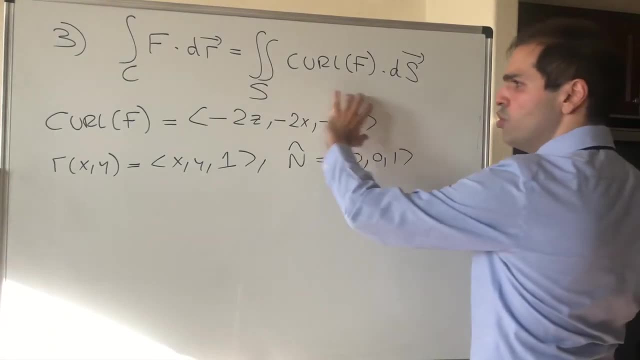 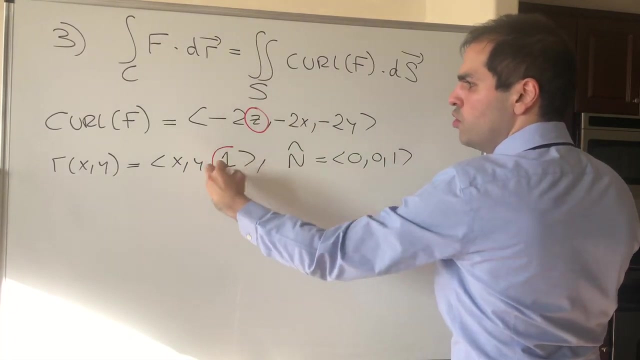 0, 0, 0, 1. so I would like to remind you how do you calculate the surface integral of a vector field? all you do, you take your vector field but replace xyz with the parametrization. so here, all you do, replace z by 1 and you dot this with the. 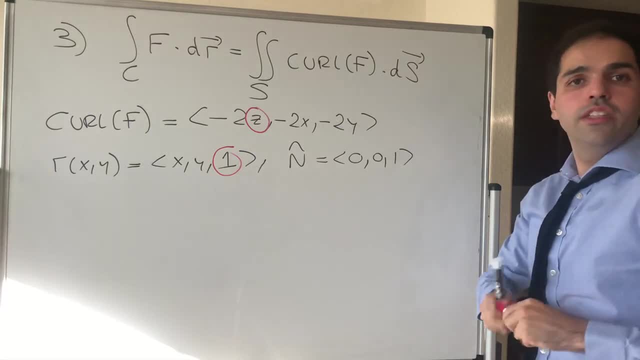 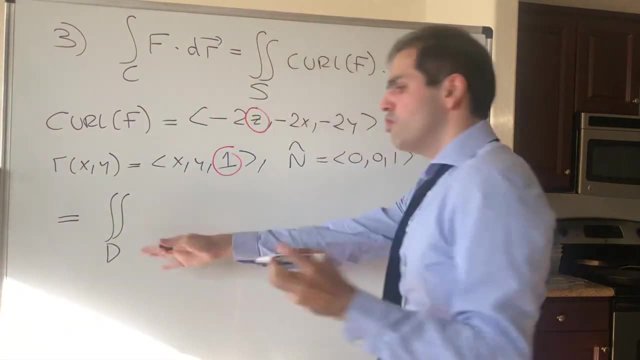 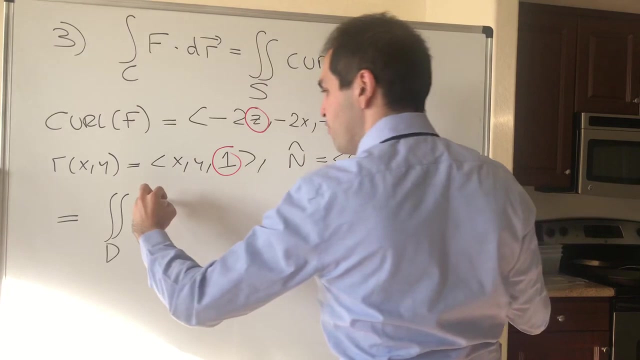 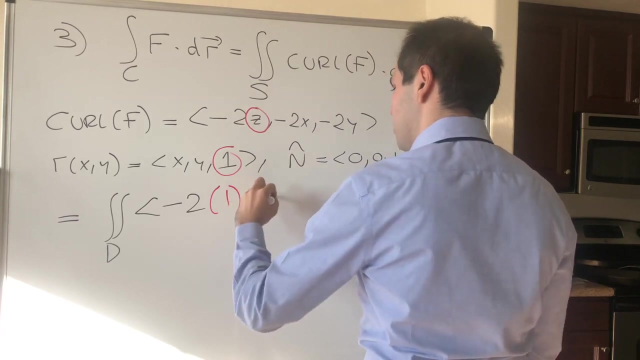 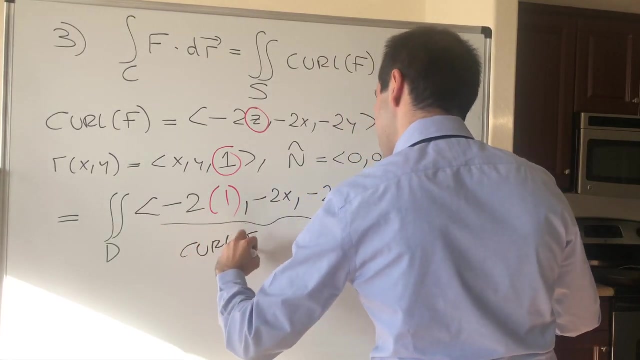 normal vector 0, 0, 1 and you integrate the resulting thing. so what this becomes is then it's the double integral over this shadow region where x and y lie in of again curl of f. but here it becomes minus 2 times 1, minus 2x, minus 2y. so again that's just curl of f, dotted with that normal vector 0, 0, 1. 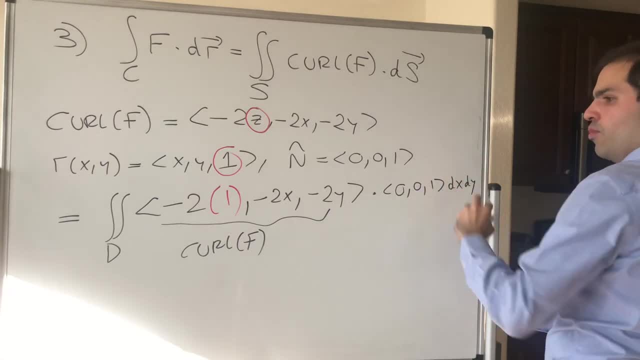 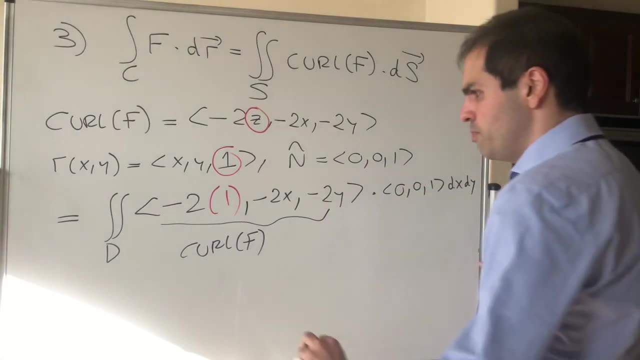 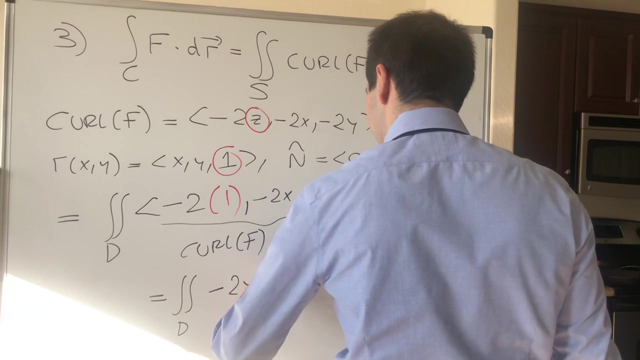 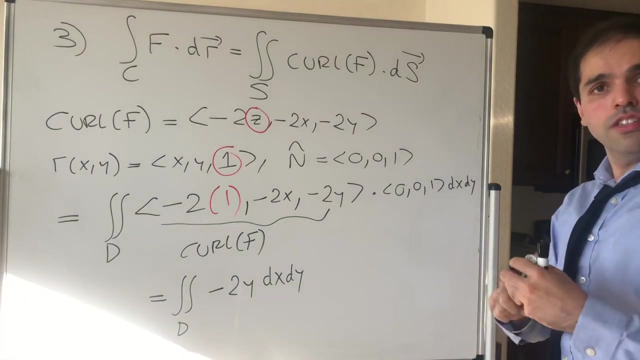 and you integrate this with respect to x and y. so the nice thing is, in the end this simplifies tremendously, just to become the double integral over d of minus 2y, dx, dy. and lastly, I would like to remind you what was d. it was just a disk centered at 0 in radius.